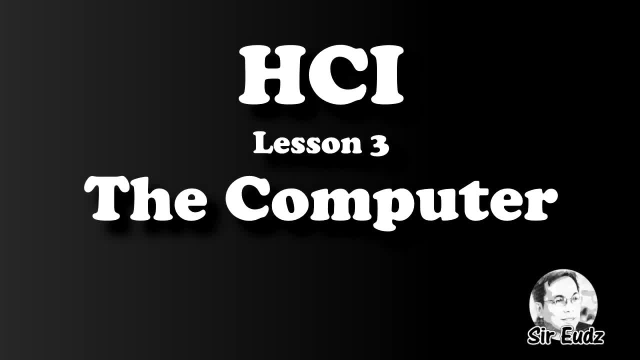 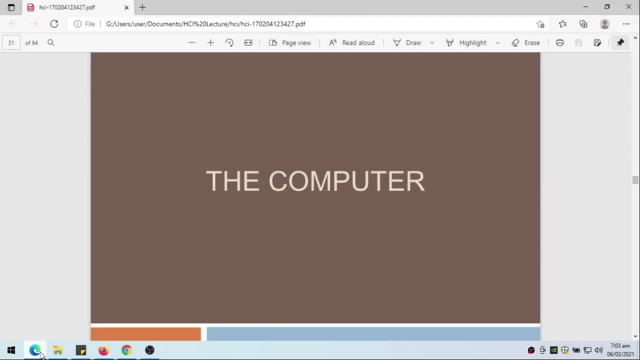 Today I'll be talking about the computer. In our previous lesson we have introduced HCI and we have more or less have an introduction of the human and how human processes, what it sees, or its input from visual audio, etc. Now let's talk about the computer. 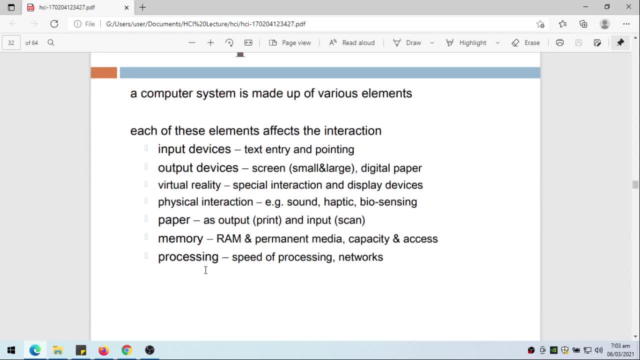 So the computer, a computer system, is made up of various elements and each of these elements affect the interaction. So some of these elements are the input devices, where we use it for our text entry and pointing. Then we have our output devices, So the screen. it can be small or large, or we can also use digital paper, etc. 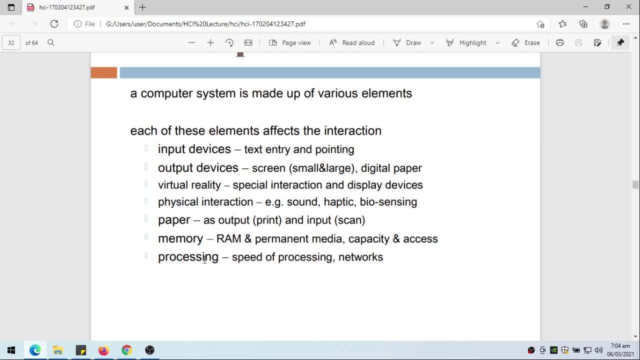 And we also have the virtual reader Reality. So it's a special interaction and display devices. We also have physical interaction, like we have the sound haptic, biosensing paper as output, print or as an input. We can scan paper memory. We have the random access memory and permanent media. 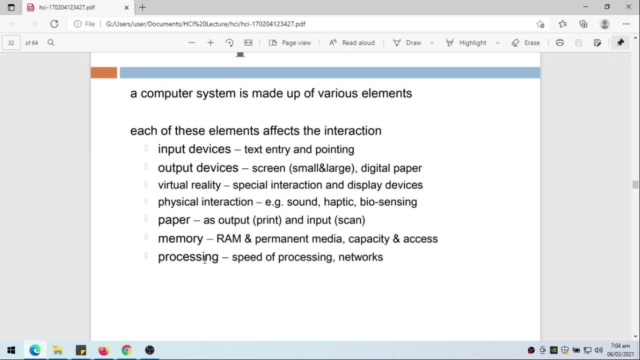 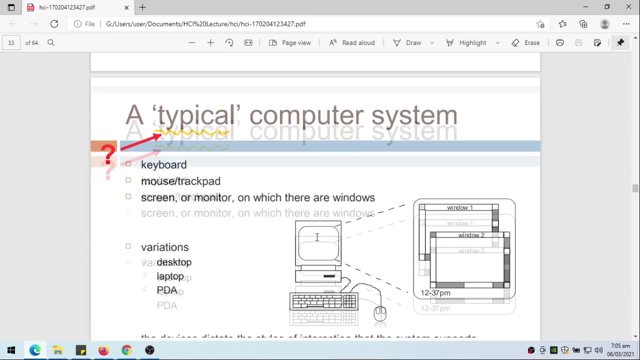 And this also is affected by its capacity and how we access data from this memory processing. So processing. We should consider this: How do we do processing? and also, how do we process data from or information from networks? Now this is how a typical computer system looks like. 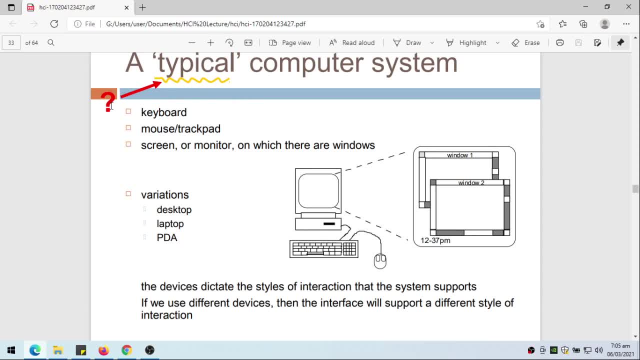 But you notice here that the typical here is we have a question mark because this is no longer maybe the typical computer system. Maybe for some we have other devices that are connected to your computer. But basically this is the What we call maybe the basic elements of a computer system. 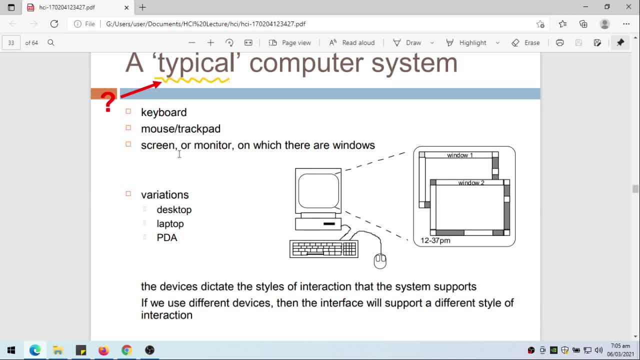 So we have the keyboard, then we have the mouse or the trackpad and we have the screen monitor, of which there are windows, especially if you're using a graphical user interface, And variations is that we can have some sort of a desktop computer, just like what is here on this diagram, here a laptop computer or a PDA, or maybe a cell phone, or PDA is what we call sometimes palm taps. 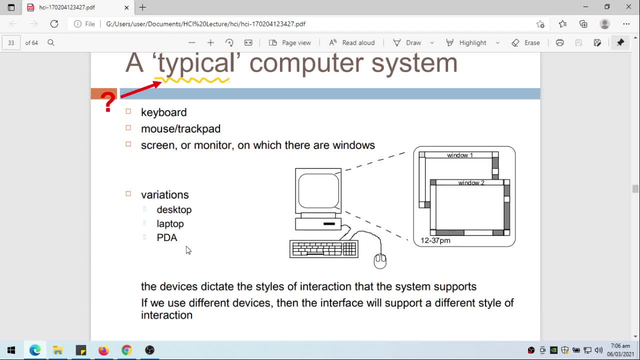 The devices dictate the styles of interaction that the system supports. If you use different devices, then the interface will support a different style of interaction. So we have a different interaction. if you use desktop, then maybe also different with a laptop, especially with its pointing devices, because sometimes laptop makes use of touch point rather than mouse, and for cell phones or palm tap computers. 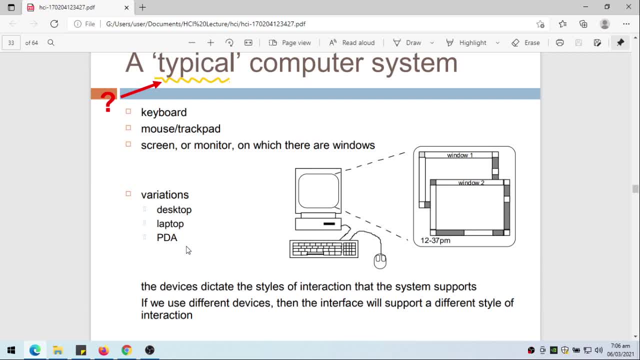 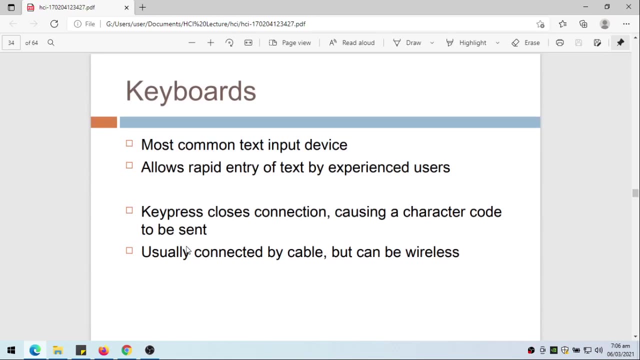 Then we could use, maybe, touch screen so we interact with these devices differently. Now here is an example of the input devices. So the keyboard is the most common text input device because it allows rapid entry of text by experienced users. So if you're an experienced typist then you can type. 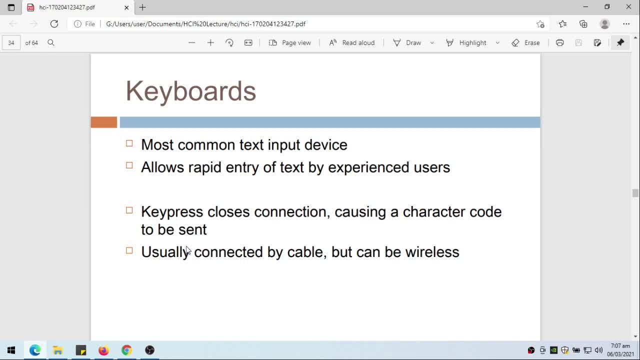 All right, Rapidly, you can enter text rapidly. So the key press. So if you press a key, actually it closes the connection and causing a character code to be sent to the computer, And usually a keyboard is connected by a cable. 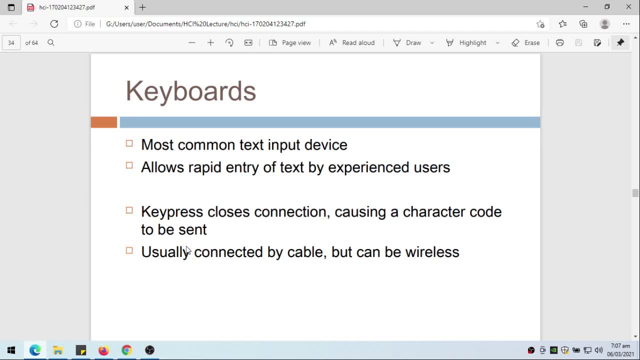 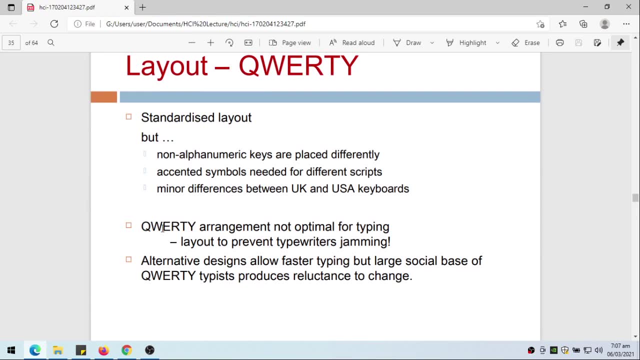 But we also have several wireless computers, maybe through infrared or through Bluetooth, And the layout of the keyboard is usually the QWERTY. So it's standardized layout, But non-alphanumeric keys are placed differently. So, especially for computers, we have the alphanumeric keys placed differently. 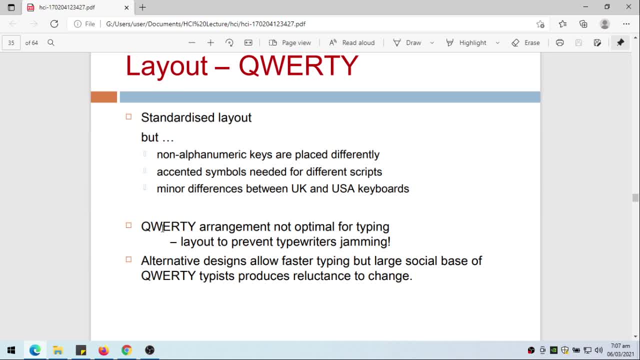 Accented symbols needed for different scripts and minor differences between UK and USA keyboards. The QWERTY arrangement is not optimal for typing because the QWERTY was designed to prevent typewriters from jamming, So that's the design of the QWERTY. 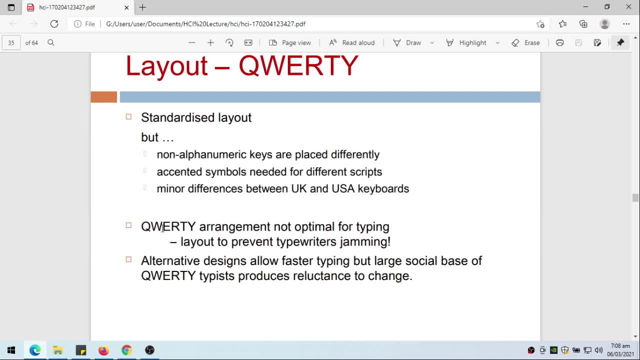 It's not really to make typing fast, but it's. the main purpose of the QWERTY layout is to prevent typewriters from jamming. So alternative designs allow faster typing, but large social base of QWERTY typists produces reluctance to change. 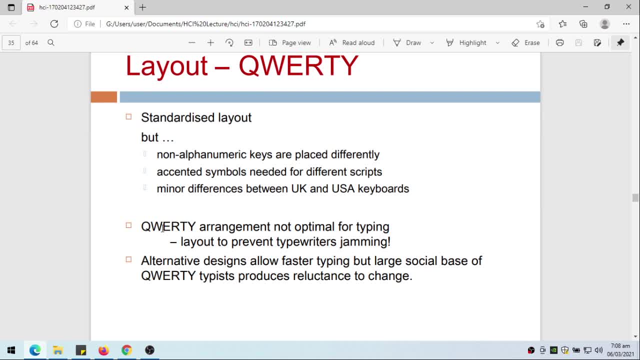 So since they're already a large social base of QWERTY typists- There are a lot of those who are using the QWERTY keyboard- Then the alternative designs could not be easily accepted by these typists. That's why, until the day, I believe that most keyboard, the layout for most keyboard, is QWERTY keyboard. 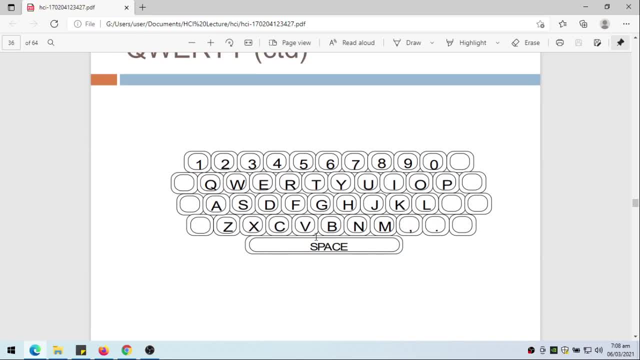 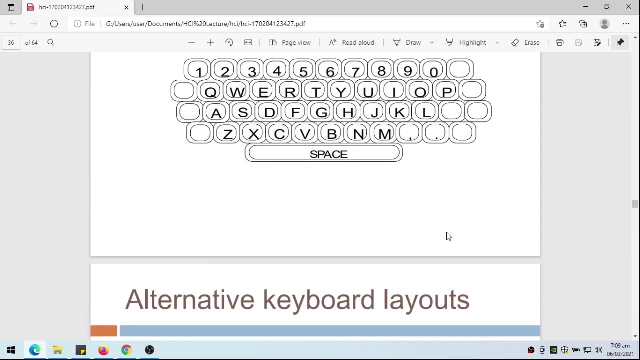 So this is the QWERTY keyboard. That's why it's called QWERTY, because on this part we have QWERTY, And most probably the layout of your keyboard is similar to this one. Now, alternative keyboard layout. 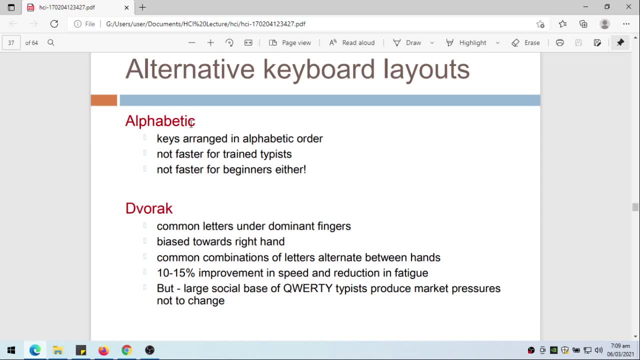 Now there are also keyboards that are alphabetic, So keys are arranged in alphabetical order, but not faster for trained typists and not faster for beginners either. So again, we also have keyboard Keyboard that are alphabetic. We also have the DIVORAC keyboard. 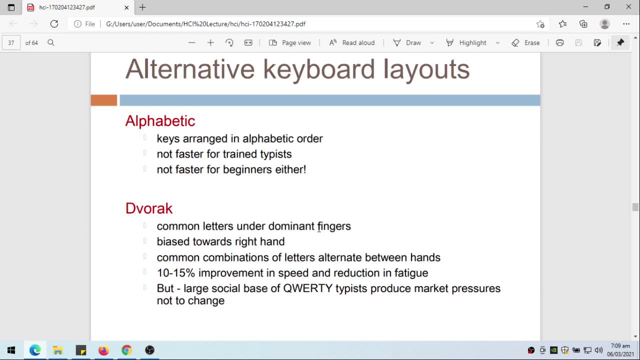 The common letters under dominant fingers. So the common letters that are used will be under the dominant finger, maybe the pointing fingers and bias towards the right hand. So more on the right hand. The most common letters are on the right hand. Common combinations of letters alternate between hands and then 10% to 15% improvement. 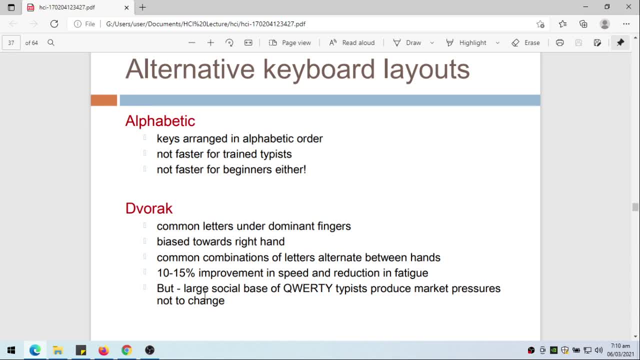 In speed and reduction in fatigue. But again, large social base of QWERTY typists produce market pressures not to change. So this is actually supposed to be a better layout of the keyboard rather than the QWERTY, But since the QWERTY has been used for quite some time now, because everything started with a typewriter. 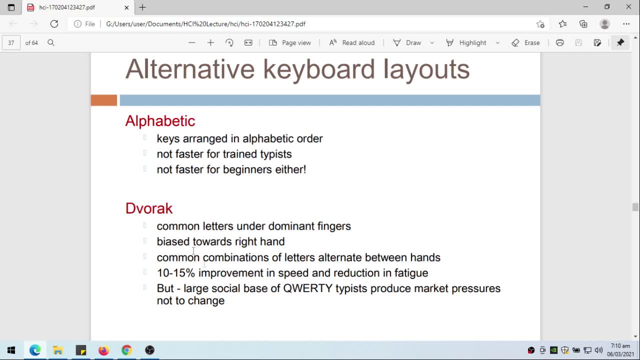 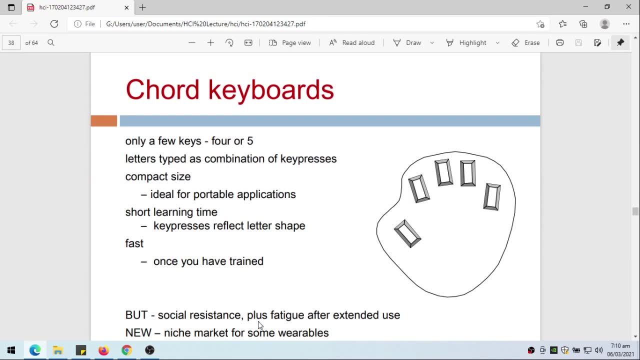 then there's a reluctance to change to the DIVORAC layout. Here's another type of keyboard, So only a few keys, four or five, And letters type as combination of key presses. So compact size, ideal for portable applications. So since it's very small, then it's portable. 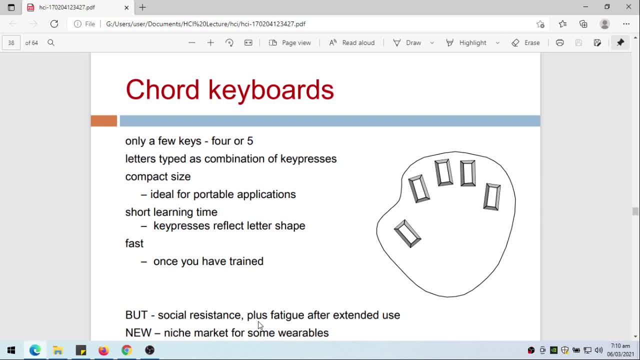 Short learning time because the key presses reflect letter shape, But I haven't tried something like this And it's fast Once you have trained. But again there's social resistance and plus fatigue after extended use, Maybe because you're only using a single hand and it's new. 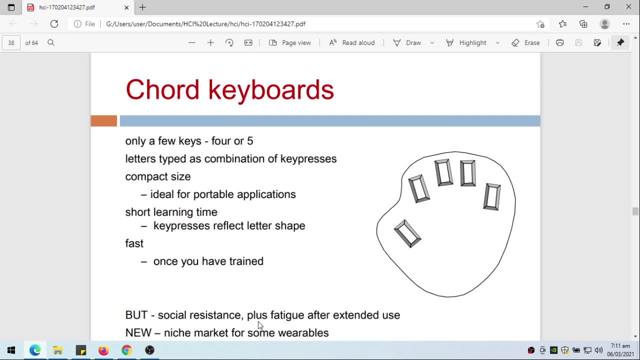 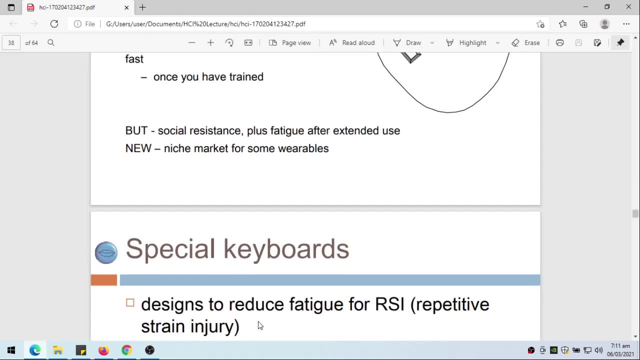 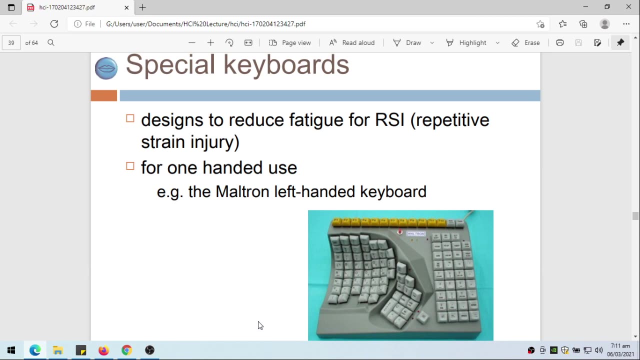 So the niche market for some wearable. So this is actually a wearable keyboard, Special keyboard, So designed to reduce fatigue, for RSI, repetitive strain injury And maybe for one-handed use. So example is the Maltran left-handed keyboard. So this is an example of a keyboard. 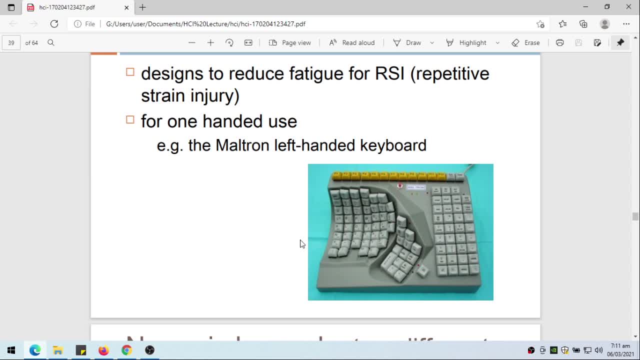 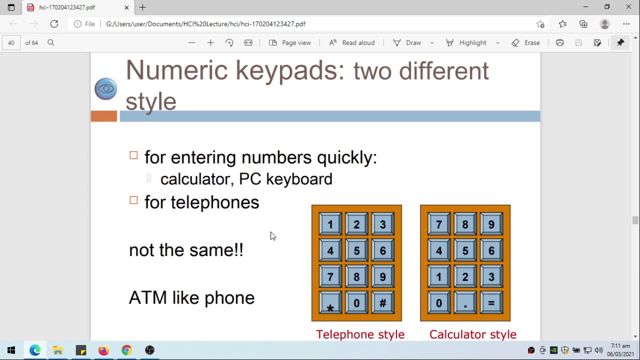 So we use only the left hand for this keyboard, especially maybe this part. Then we also have numeric keypads And maybe, if you haven't noticed yet, there are two different styles for entering numbers quickly: Calculator, PC keyboard. It's quite different with that of the telephones. 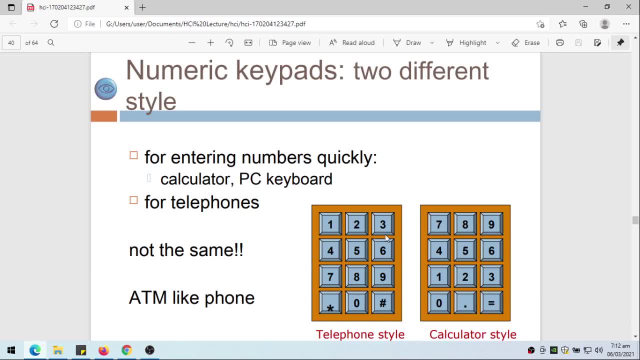 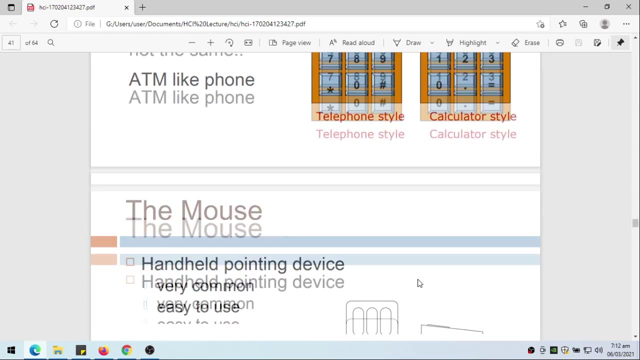 So not the same. So for telephone the numbers one, two, three are on the top, While for calculator and keyboards numbers one, two, three are at the bottom. Then the mouse. So the mouse is a handheld pointing device. 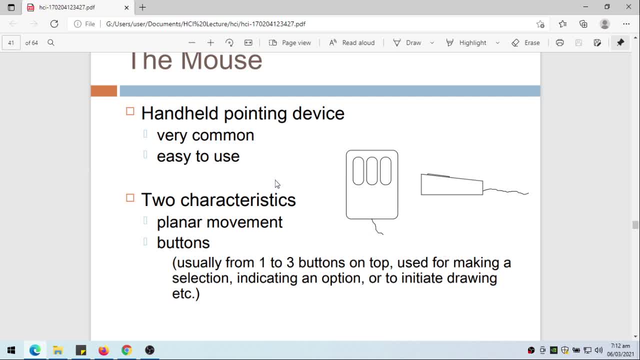 And it's very common because it's easy to use. There are two characteristics, So the planar movement, So the movement is interpreted, And also the buttons, So usually from one to three buttons on top used for making a selection, indicating an option or to initiate drawing, et cetera. 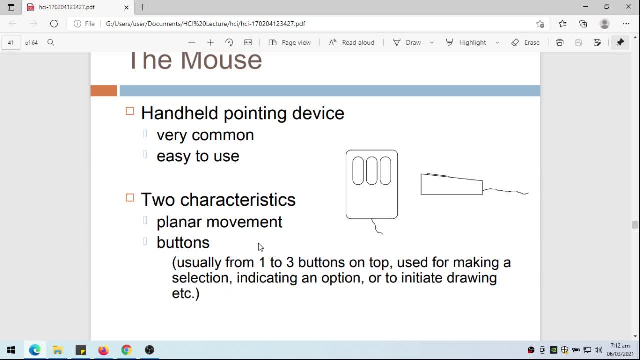 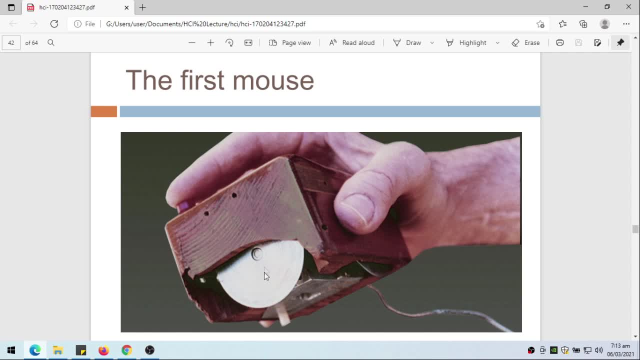 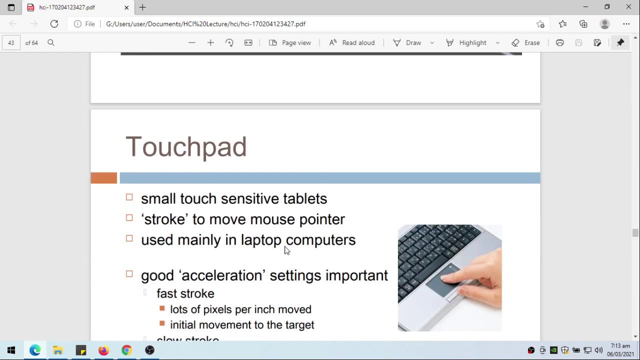 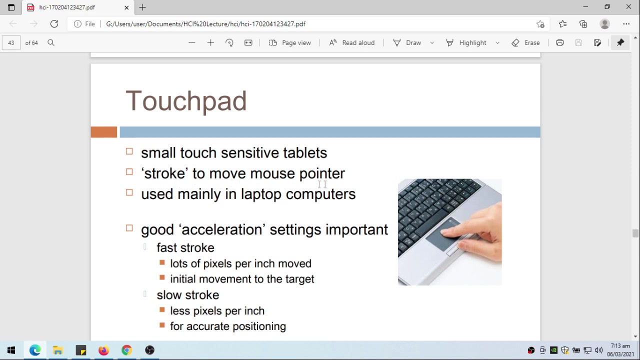 So more or less you're familiar with the mouse. Now, if you're quite interested, this is how the first mouse looks like. Okay, Then we also have the touchpad. Touchpad is small touch, sensitive tablet stroke to move mouse pointer and used mainly in laptop computers. 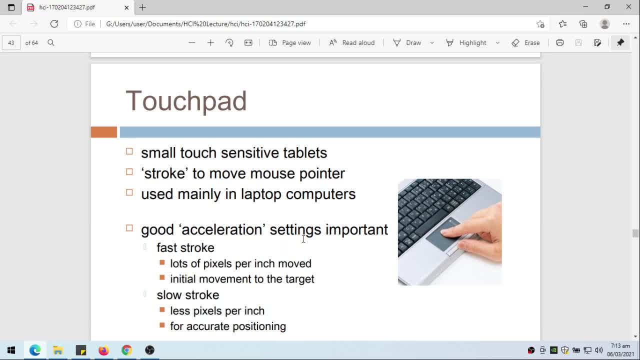 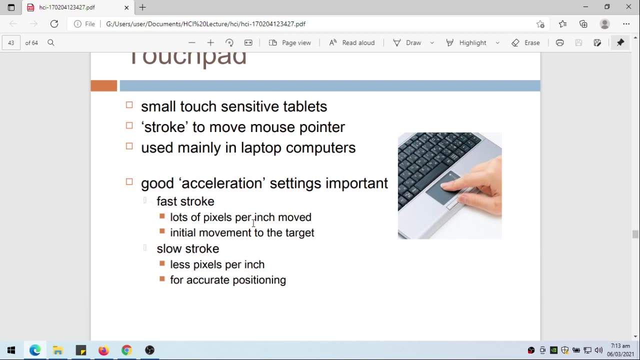 So it has good acceleration settings. if you have the correct settings And then fast stroke, So a lot of pixels per inch move, initial movement to the target. Slow stroke, Less pixels. So if you use fast stroke, lots of pixels Per each. 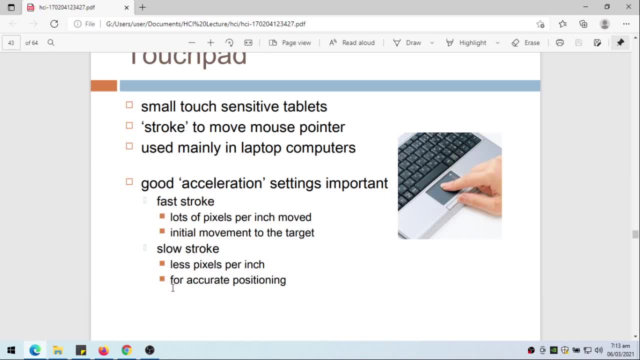 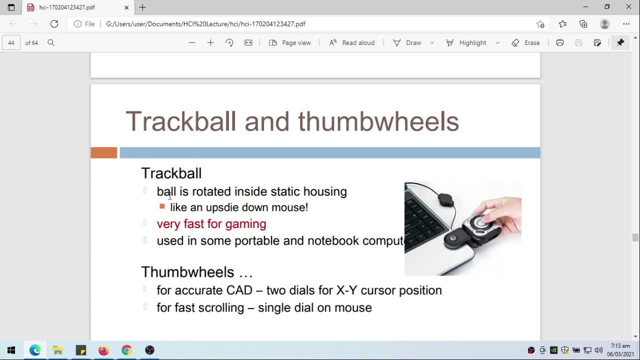 So if you have slow stroke, less pixels per inch, This is used for accurate positioning. Then we also have truck balls and thumb wheels. So truck ball, The ball is rotated inside static housing like an upside down mouse. It's like a mouse, but it's upside down because the ball is actually on top, especially the older mouse. 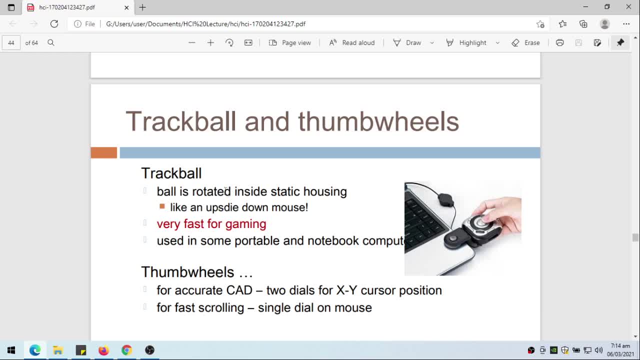 We have the mechanical mouse. We have actually some sort of a ball At the bottom of the mouse, But here it looks like an upside down mouse, So that ball is actually on top. So very fast for gaming, Used in some portable and notebook output. 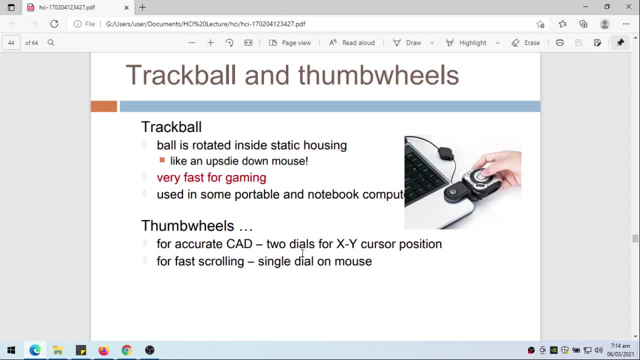 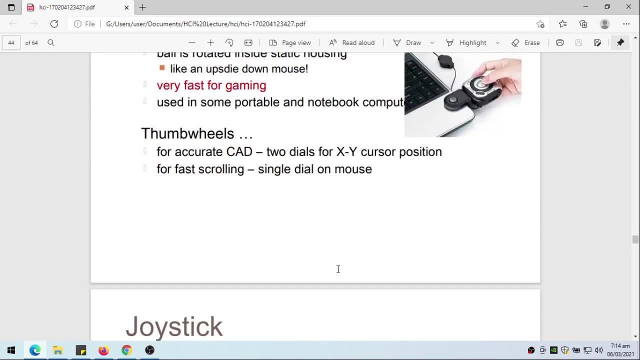 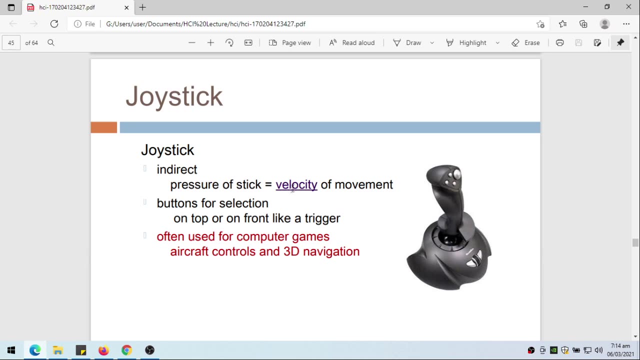 We also have thumb wheels for accurate CAD, or two dials for XY cursor position for fast scrolling, single dial or mouse, Then joystick. We also have the joystick, So indirect pressure of stick, Velocity of movement, So buttons for selection. So we have on top or on front trigger. 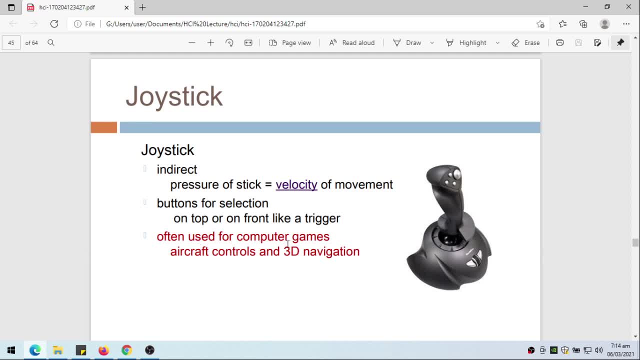 So these are the buttons for selection. They are often used for computer games and aircraft controls in, like aircraft controls in 3D navigation. So this is an example of a joystick. Now let's talk about memory, So the short term memory of computer. 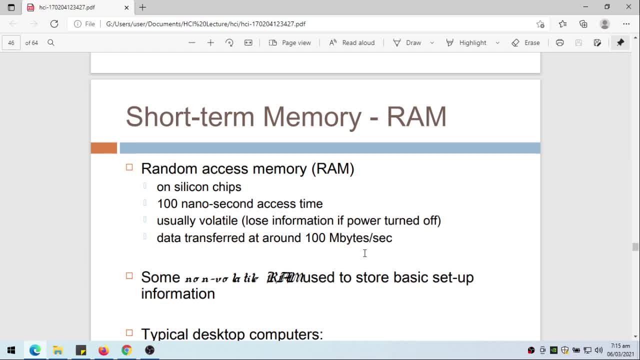 We actually make use of the random access memory. So the random access Memory is, of course, placed on silicon chips and 100 nanosecond access time- maybe even faster now- usually volatile. So that means you lose information if power is turned off and data transferred at around 100 megabytes per second. 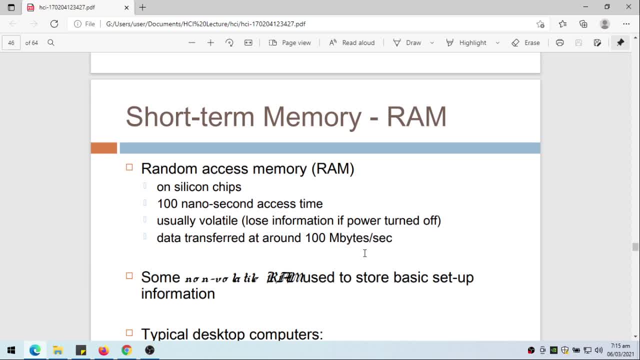 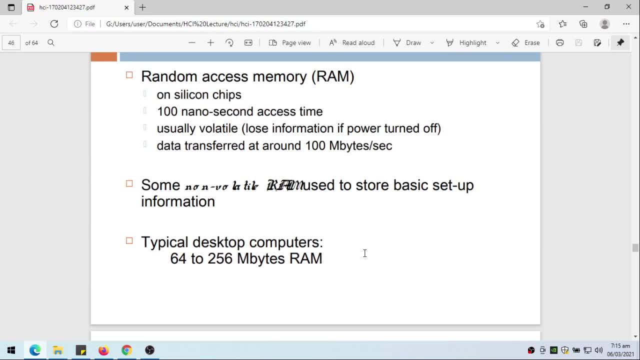 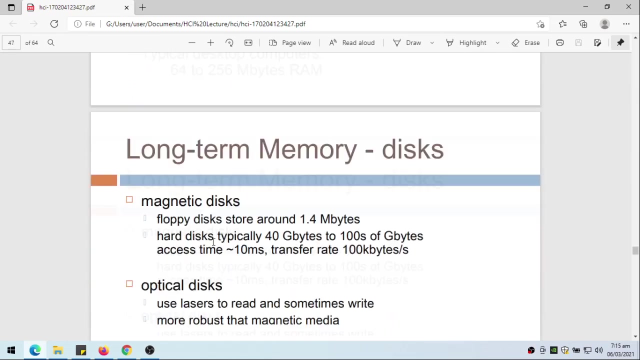 Some non volatile ROM used to store basic set up information. So typical desktop computers have 64 to 256 megabytes of RAM. I think this is already false. So we have gigabytes of RAM already. How about long term memory? So for long term memory we actually make use of the disk. 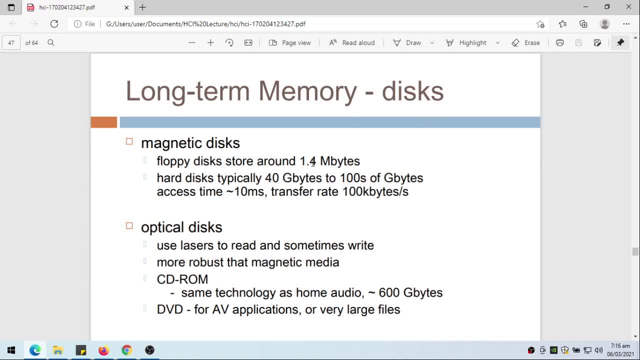 So like magnetic disk, So floppy disk store around 1.4 megabytes. Hard disk, typically 40 gigabytes to 100 gigabytes. It's no longer true. We have now terabytes of hard disk access Access time is approximately 10 milliseconds. 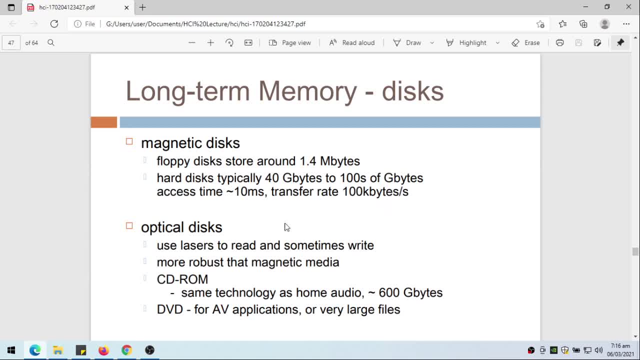 Transfer rate is 100 kilobytes per second Optical disk. So these are the CDs et cetera. So use lasers to read and sometimes write, and more robust than magnetic data and CD ROM. Same technology as home audio, So approximately 600 gigabytes DVD for AV applications or very large files. 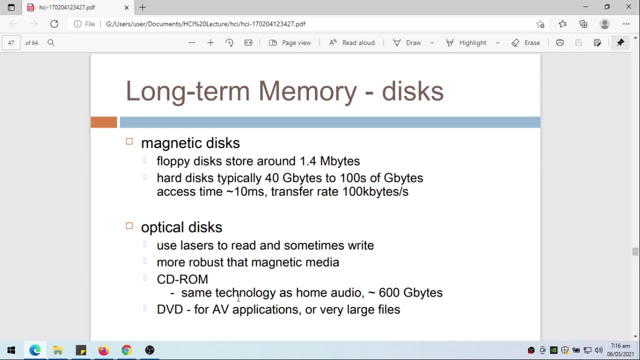 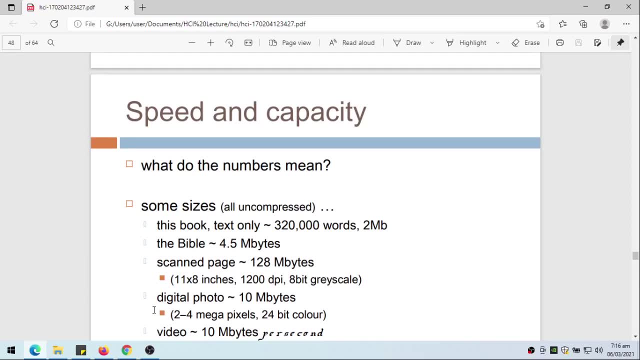 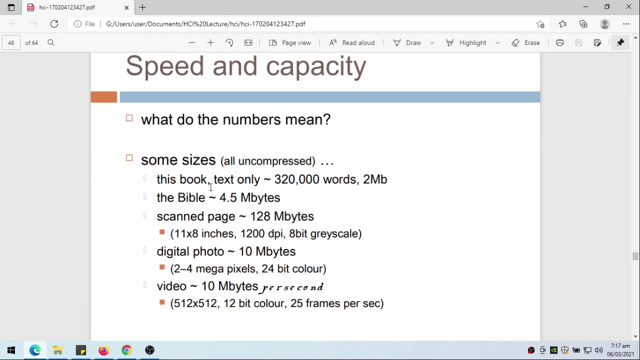 Now we usually- we now use this rarely already- Speed and capacity. What do these numbers mean? So some size set. So this book- I know we're not using a book, so maybe a typical book. I have 312,000 words, so that's around two megabytes. 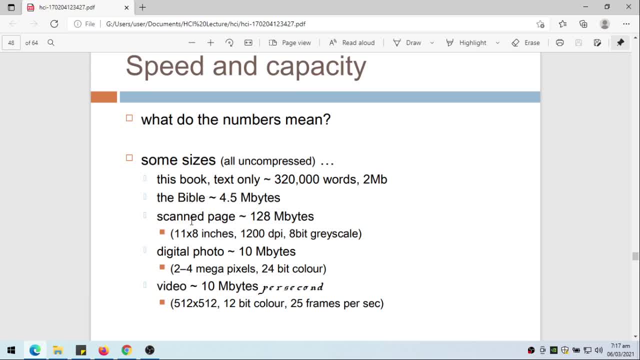 The Bible is around 4.5 megabytes. Scan page is around 120 megabytes, but that's 11 by 8 at 1,200 dots per inch and 8 bit gray scale. But of course if it is colored it will be a lot bigger. 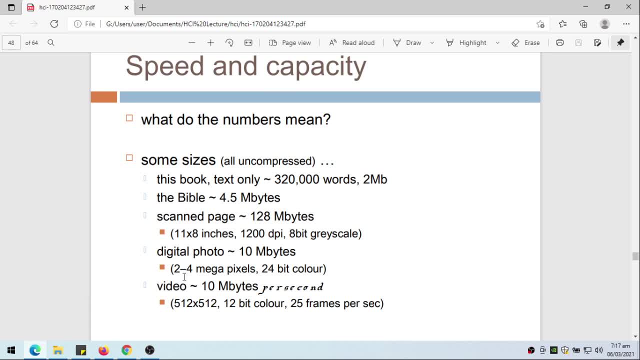 Digital photo, That's around 10 megabytes. That is if you're using two to four megapixels and 24 bit color. But of course now it's even bigger video: 10 megabytes per second. That's using 512 by 512, 12 bit color and 25 frames per second. 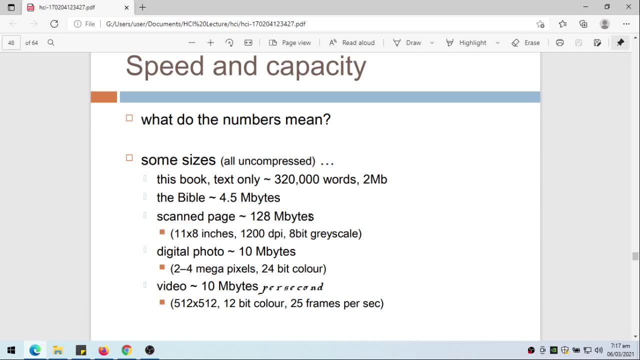 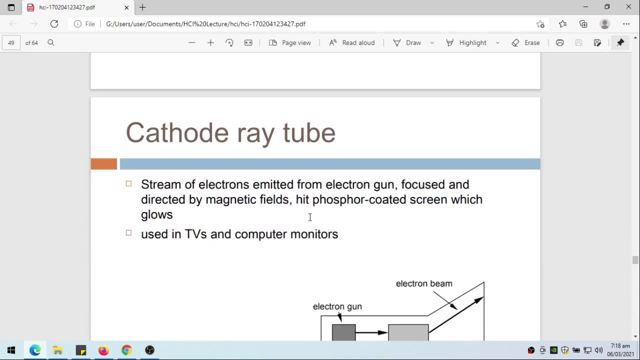 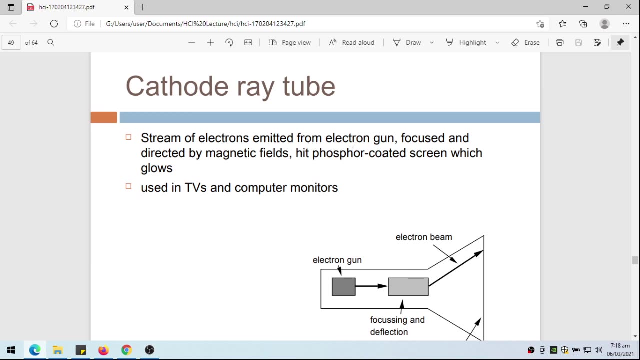 And again this is no longer true, So these are already old values. Excuse me, The cathode So a stream of electrons emitted from electron gun, focused and directed by magnetic fields. So heat phosphor coated screen which glows. 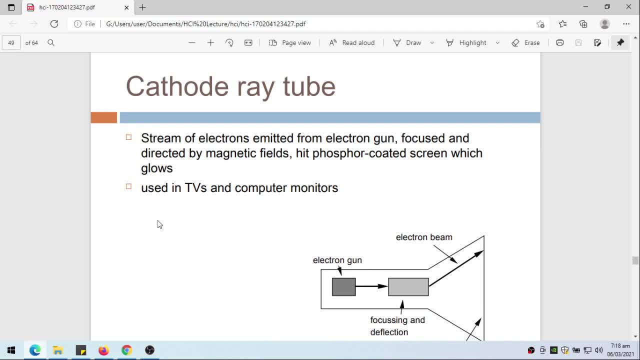 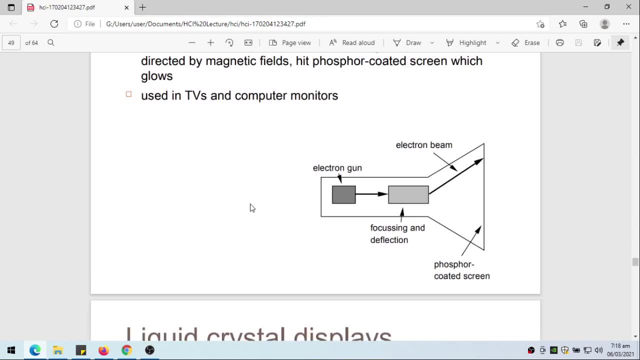 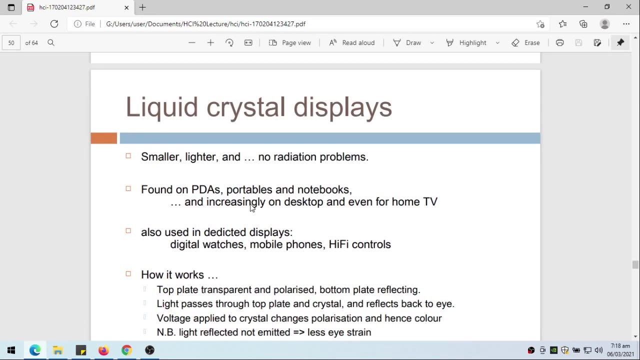 So this will hit the screen and then the screen will glow. So using TVs and computer monitors. Then we have the liquid crystal displays And of course, lately we have not only LCDs but LEDs. so smaller, lighter and no radiation problems found on PDAs. 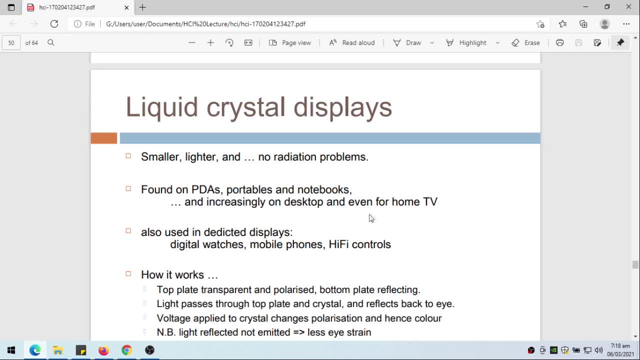 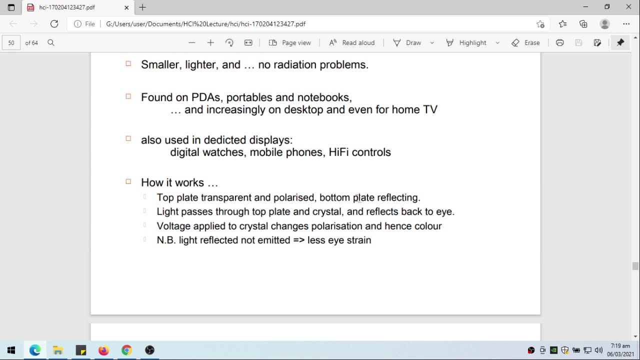 portables and notebooks and increasingly on desktop and even for home TV. But actually now it's already the standard, Also used in dedicated displays like digital watches, mobile phones, Hi-Fi controls. So how it works: Top plate transparent and polarized. bottom plate reflecting. 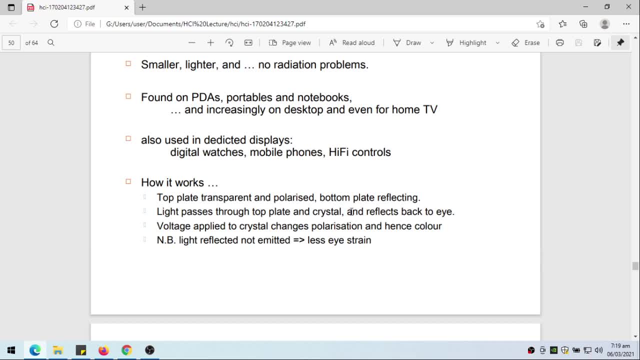 So light passes through the top plate and crystal reflects back to the eye. The voltage applied to crystal changes polarization and hence color. So light reflected, not emitted, So there is lesser eye strain as compared with the cathode ray tube Now in printing. 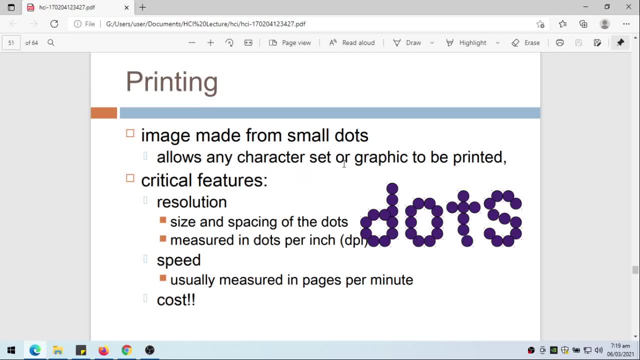 image made from small dots, so allows any character, set or graphics to be printed. So the printing is something like this: It is composed of several dots. So critical features for printers. We have the resolution, So the size and spacing of dots, measured in dots per inch. 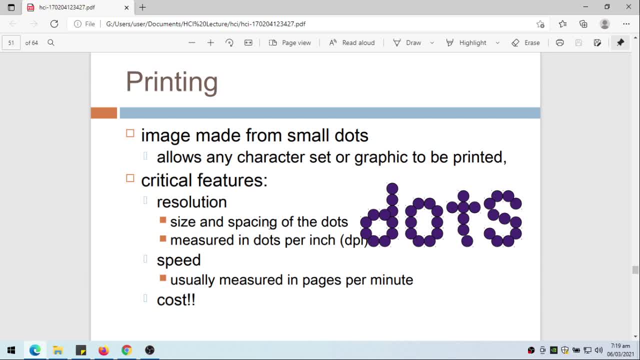 So the higher the dots per inch, then that means the better is the resolution and the better is the appearance of the text. The speed is usually measured in page per minute And of course sometimes this is affected by the cost. Sometimes the faster. 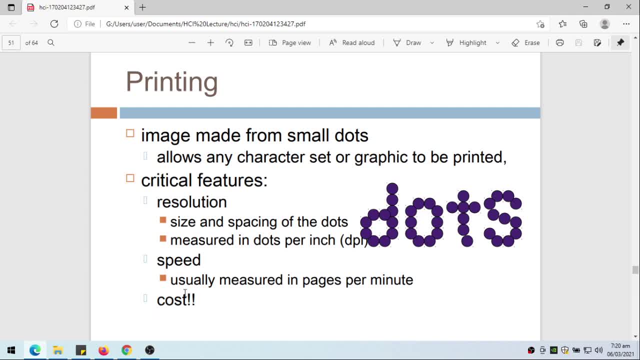 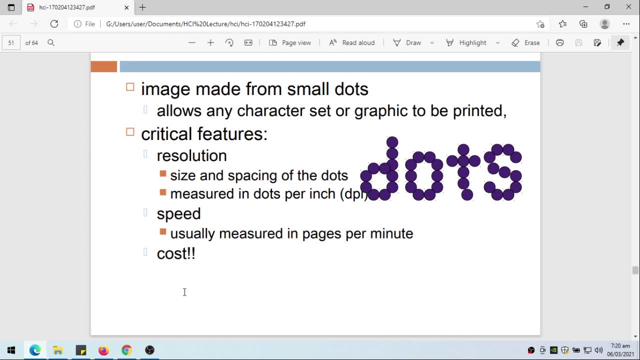 The computer. the better the resolution is, the higher the cost. So actually this is just a some sort of a review of the devices that are used for, but used by the computers, So for input and output. So there are other devices and maybe we'll.